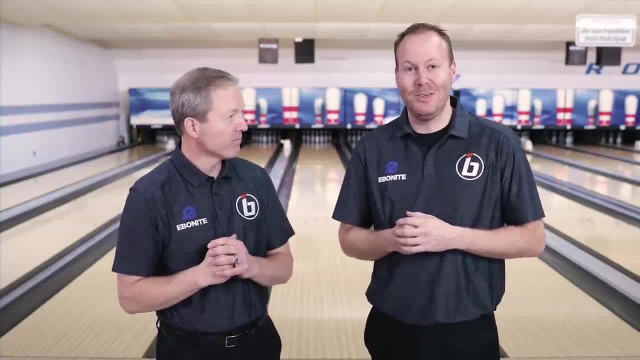 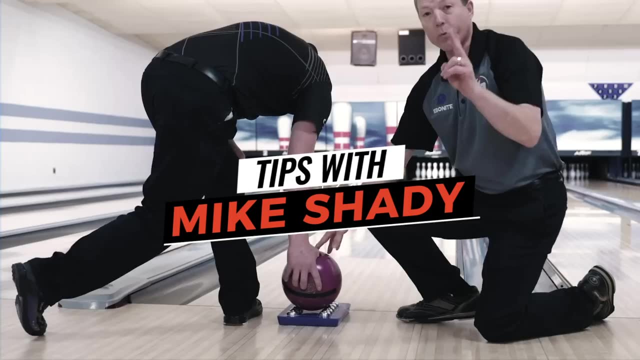 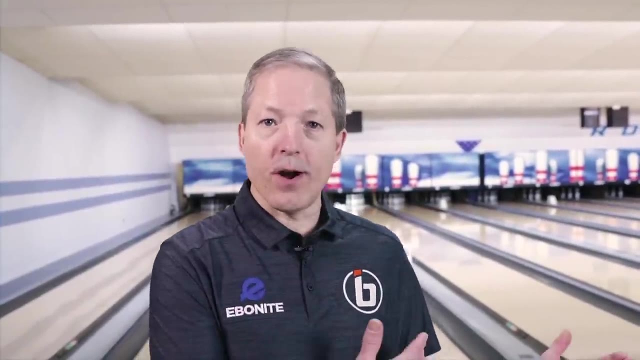 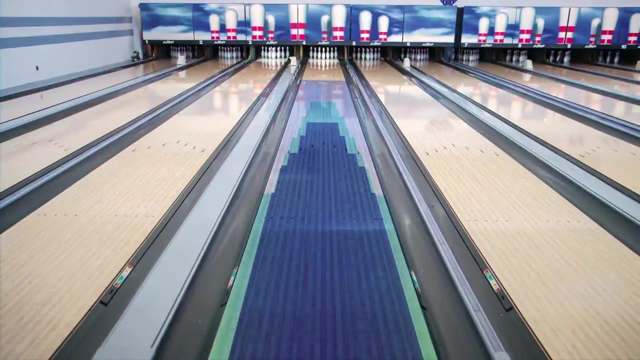 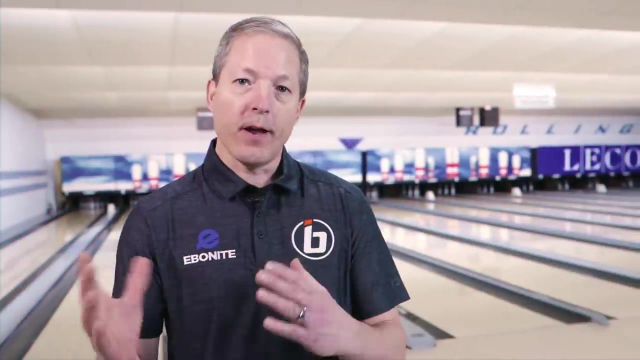 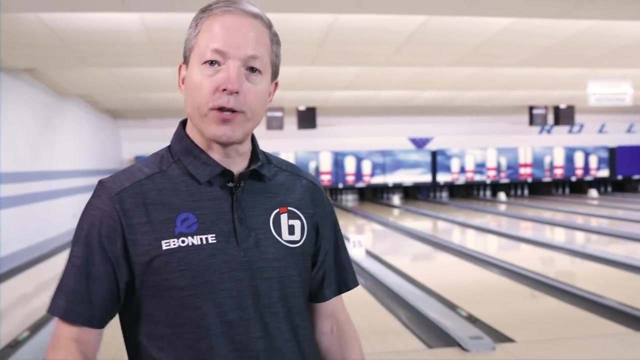 All right. Well, I'm going to stop talking. I can't wait to see this. Let's go out and see what one shot looks like. One Shot, One Shot. One of the greatest challenges in the sport of bowling is the environment we play in. We have what's called lane conditioning or, as we call it, oil that's applied to the lane but it's invisible. You can't see where it's applied. You don't know how far it goes down the lane. So today I want to determine some that help you out on how to play the lanes, to make the game much more easy. If we look out in the lane, I've got three markers: a 15,, a 35, and a 45 marker, And, as the 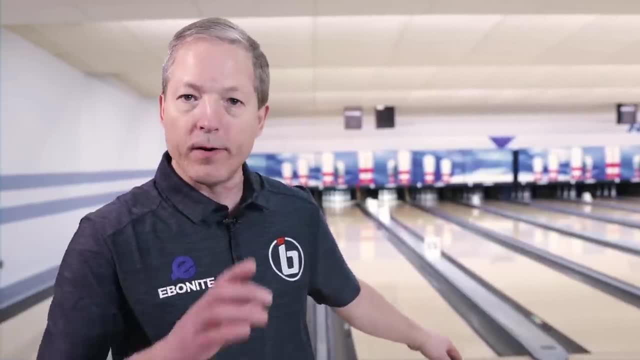 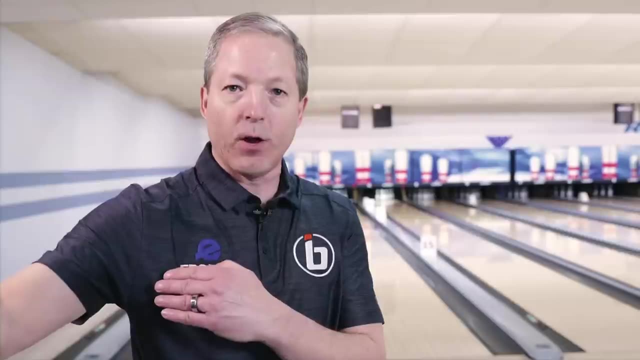 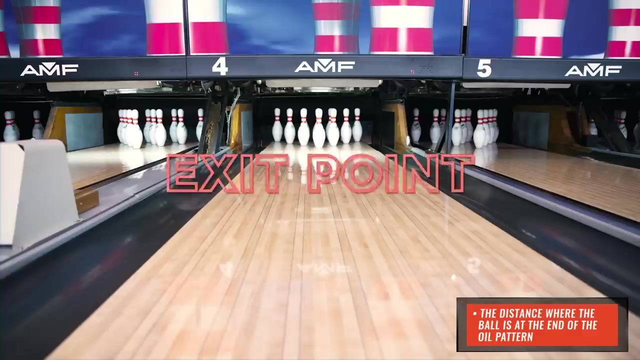 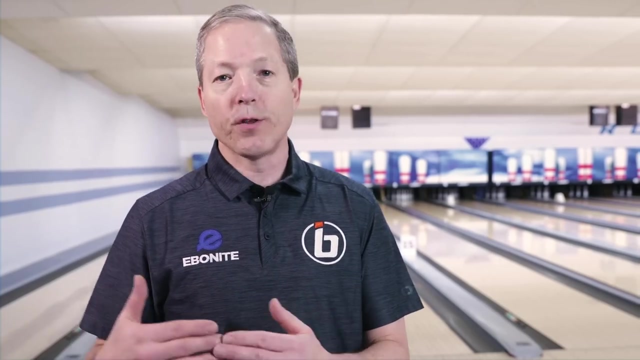 lane is conditioned or oiled for the player to make the environment either easier or more difficult. it's oiled from the front to the back, but there's a stopping point of the oil And we call that the exit point of where the ball starts to hook toward the pins. Today, I want to determine how do we figure out that exit point, because that's the secret formula of how to play lanes. Most of the oil today is stopped around those different distances. First of all, 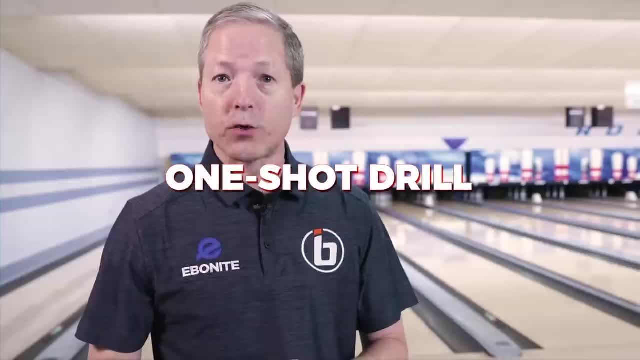 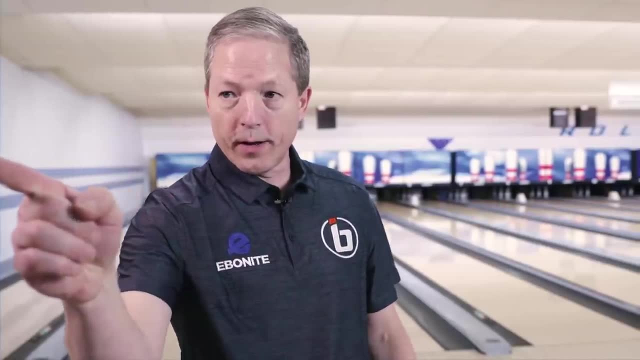 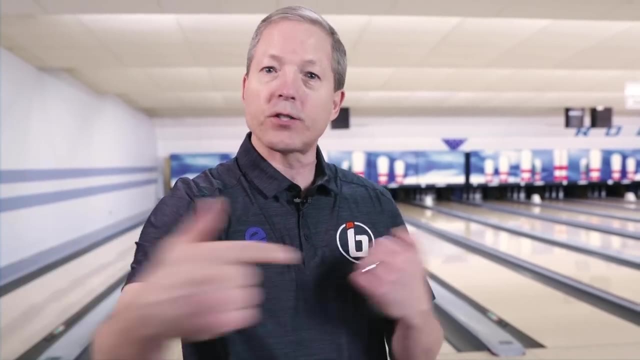 I want to show you is. I'm going to give you a small drill- It's called a one-shot drill- on how to determine where the play, and I'm just going to go up there and spin the ball And when it starts to go down the lane, as soon as it makes its break point, we've determined, from the foul line to that exit point, the distance of the oil. Let's take a look. 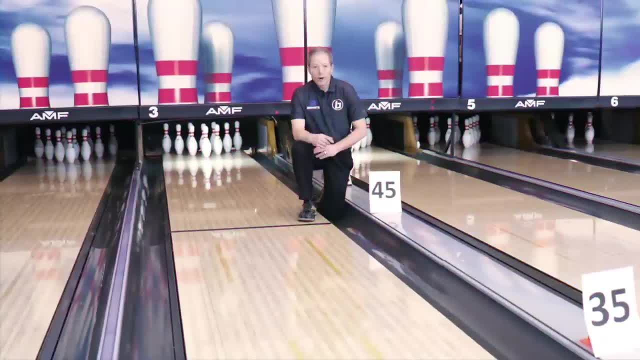 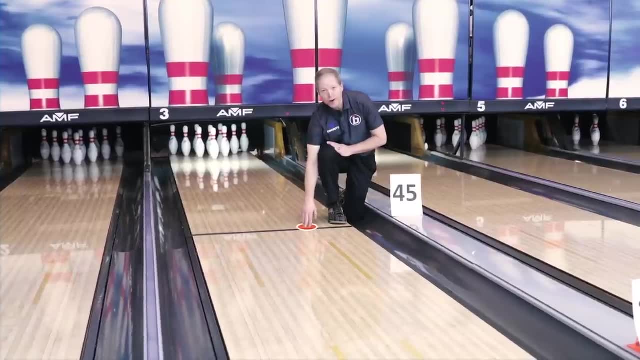 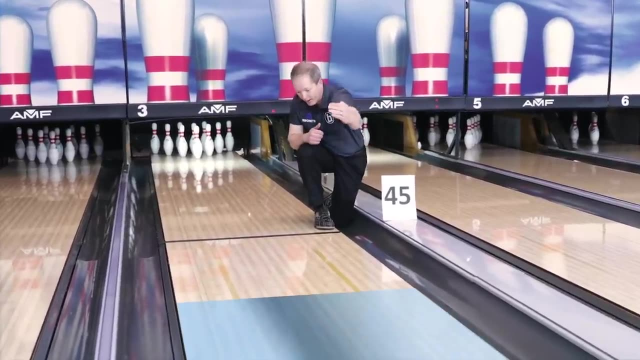 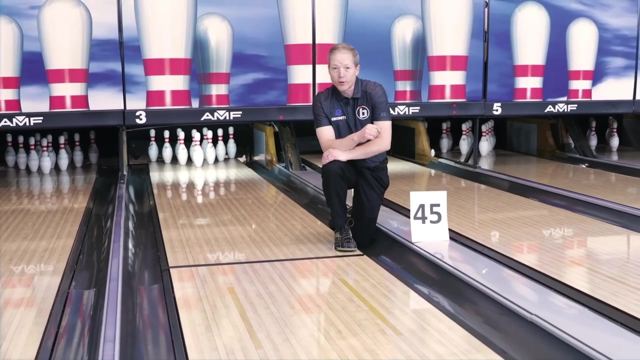 So, as you could see, as the ball made its move, it's started to hook right around this spot here. This is the 45-foot mark. This is where the oil ends on the lane, So the invisible environment. we've got oil from the foul line right to this spot, which is 45 feet. Now, in bowling we have a formula that was developed several years ago and it's the distance of the pattern the oil where it starts to hook. 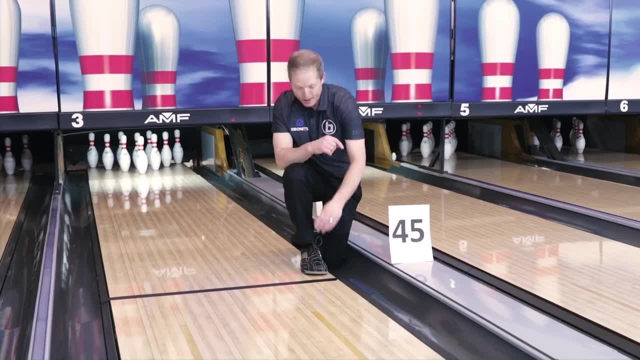 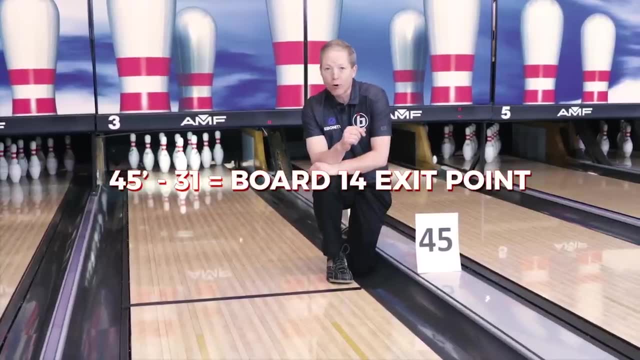 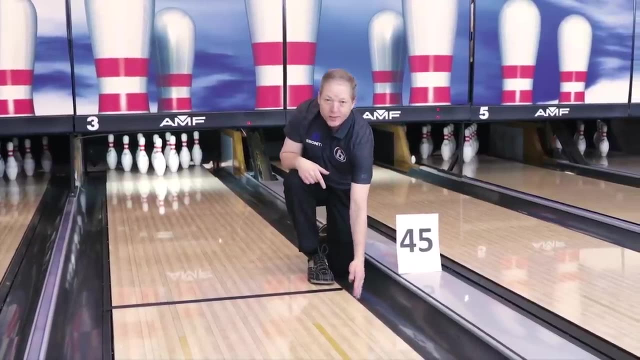 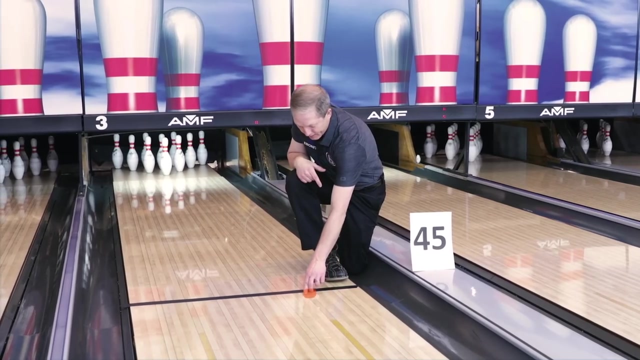 So we've got about 45 feet, as you can see our markers. If we subtract 31 from that, we're at about board 14 for the exit point. Now what that means is this is board one. It's the board right next to the gutter. So if we count 14, we're going to be- we've got 3,, 4,, 5,, 6,, 7,, 8,, 9,, 10,, 11,, 12,, 13, 14.. So we want the ball to break right around this spot here. 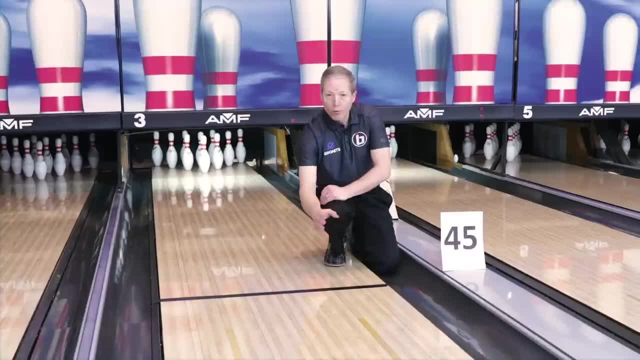 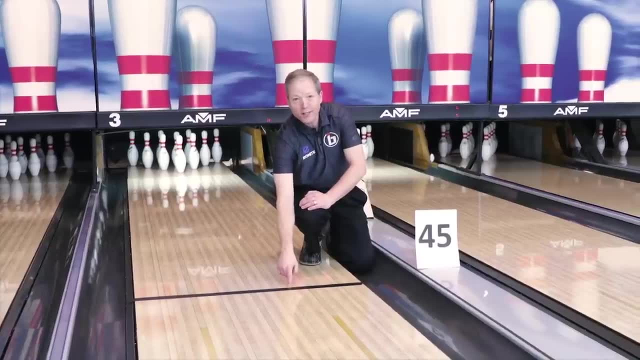 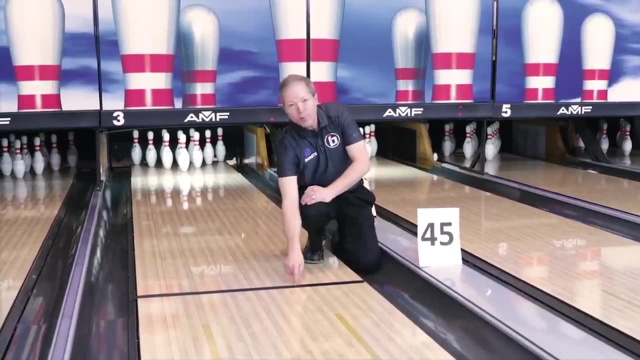 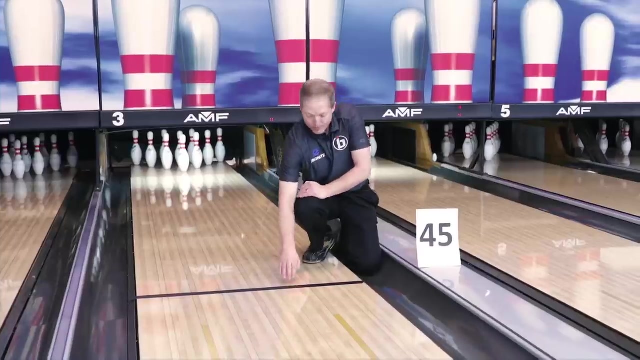 Now it could be one or two boards left or right of that, depending on the surface, but this is my goal as I start my practice session. after that, one shot on how to get lined up. I want the ball right in this area, at my exit point, as it starts to make its move to the strike pocket, to get lined up. This is the secret formula on how to get to the strike pocket. 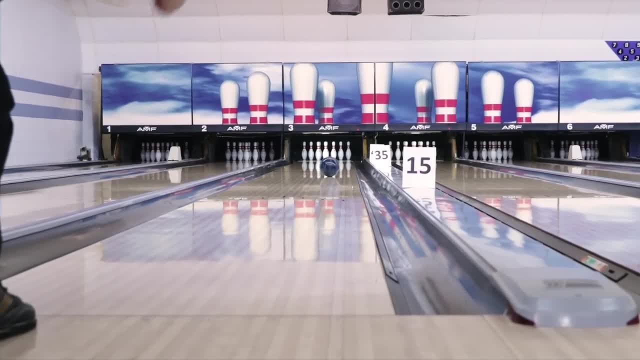 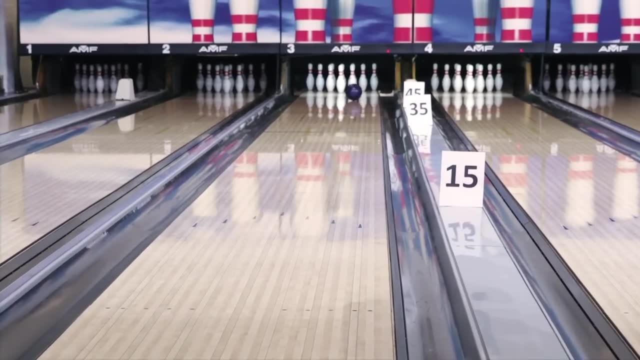 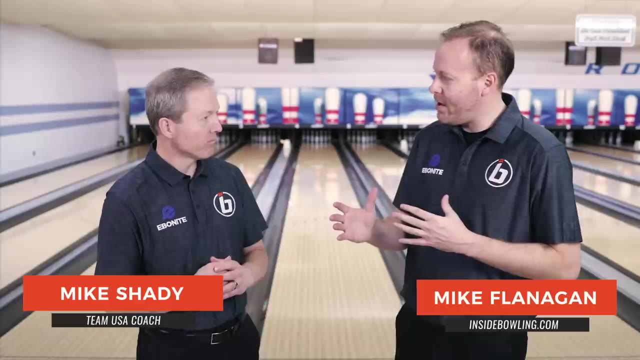 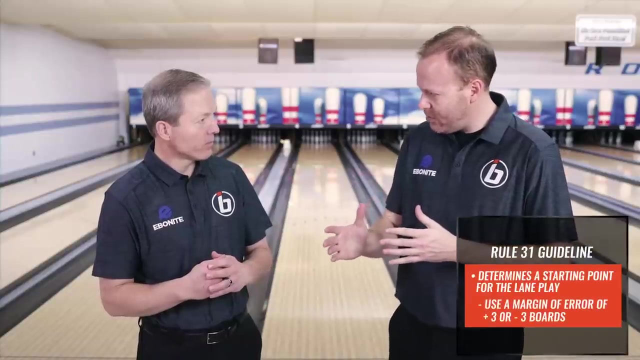 And score it your highest. Seeing that ball change direction down the lane and that one shot throwing it nice and slow, you really get to see where the break point is. But I do want to ask a question to follow up after watching the video there: Do we want to take the rule of 31 literal and is it the exact board out there? 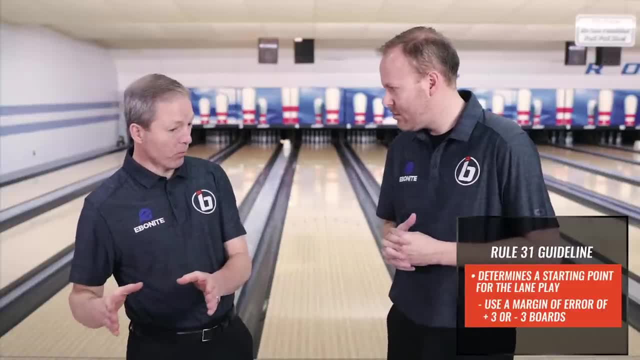 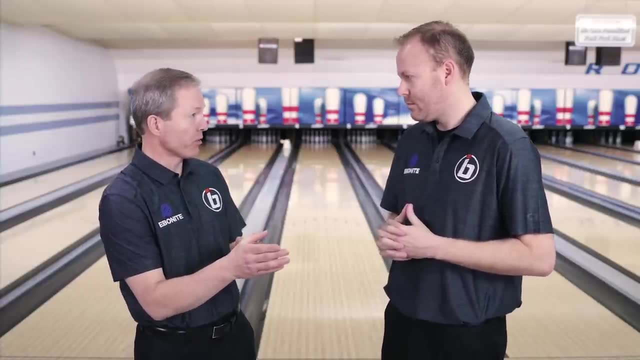 No, it's a starting point, Mike. But again, our goal here Was how do we make every shot count So it gets us closer to the area I like to build in? plus or minus three lanes are all different. You know, a Brunswick versus an AMF, You know one's one's a little slicker than the other, The type of oils, the machines, the age, the all of that takes in consideration that plus or minus three. So it's a starting point, but I really believe it minimizes the number of shots we waste to try to figure out what we're going to do next. 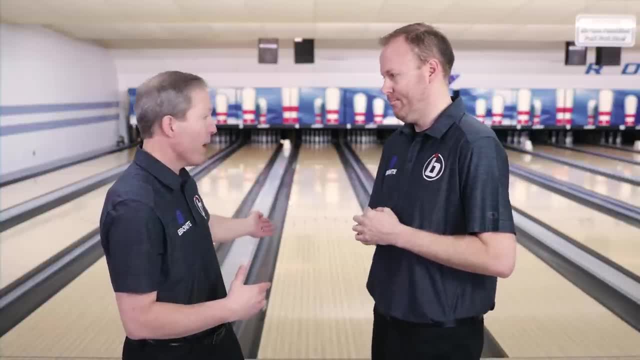 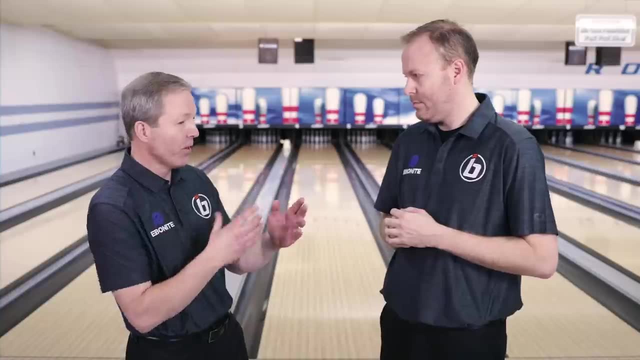 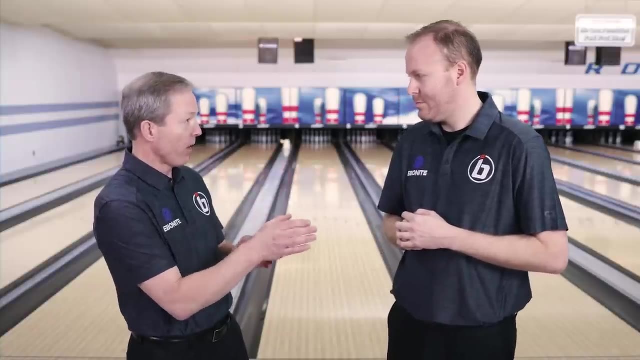 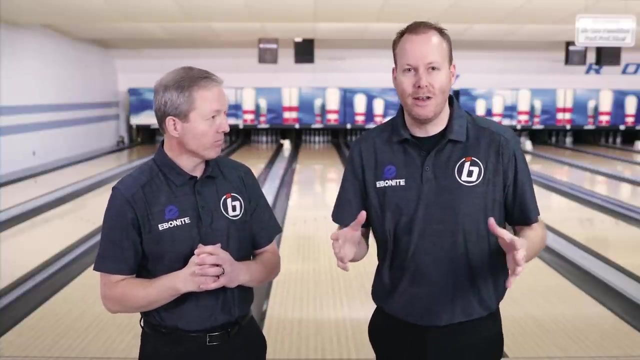 So I think it's a starting point, But where the exit point is at the end of the lane, Absolutely. So we want everybody out there to start this worldwide. Your very first shot in league or tournament. Just walk up there, See how long the pattern is.